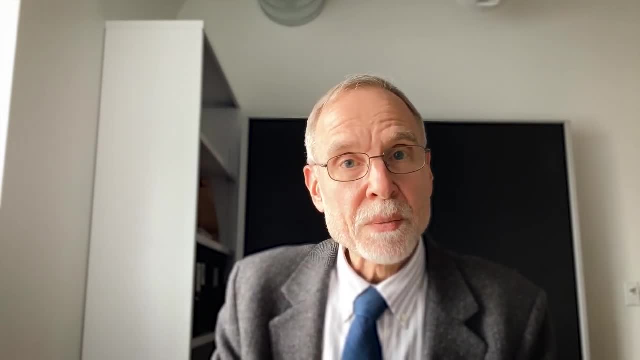 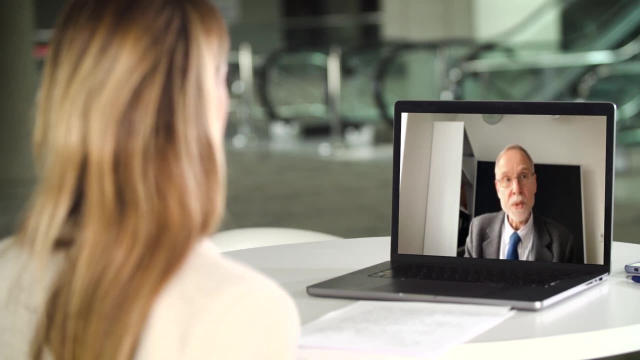 Also, I think every paper I read has some modeling and simulation, Even if it's in the supplementary information. that paper could not get published without it and my students realize that and they know that they need those sorts of skills. I think modeling and simulation is very good for developing intuition and for developing an insight into what questions should be asked and what experiment needs to be done. 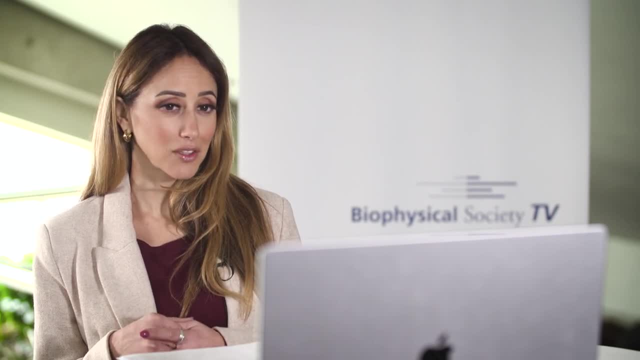 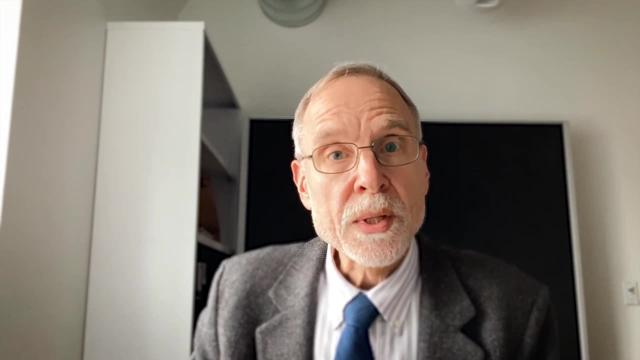 Now, are students with little computer experience still able to excel in your class? Every time I teach my class on the first day, I ask them to self-report. I ask them to self-report on their computing skills and how much coding they've done, and about half the class says zero. 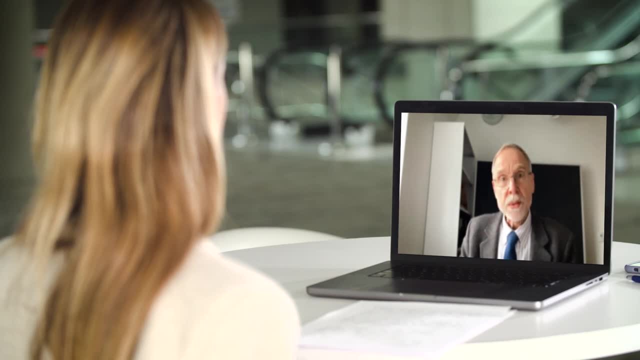 Yes, they are able to excel. We bring them up to speed. We have found that Python is a language that they can get up to speed pretty quickly and we can just add a little bit every week And to them. it's so much more exciting than just taking a computer science course where everything is done in the abstract. 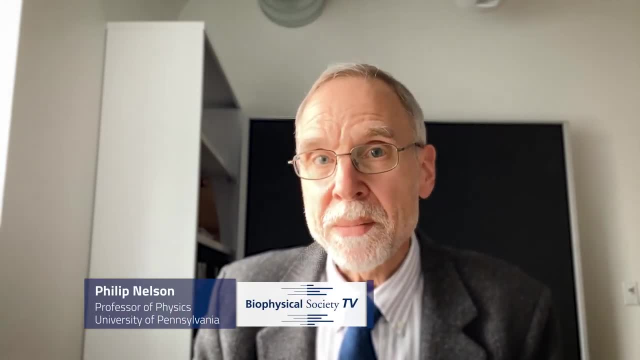 It's good to know how to make a graph, It's better to know how to make an animated graph, because animated graphs have a plot line, They tell a story And as you go along, you're going to learn a lot. You're going to learn a lot. 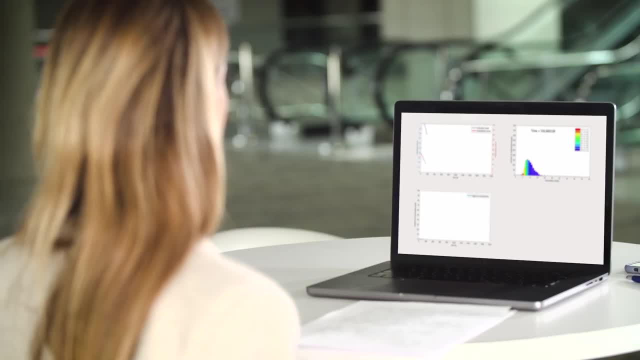 As you can see in the animation that I'm showing right here, I personally never really understood adaptation and bacterial chemotaxis until I made this little simulation and turned it into an animation and watched the storyline. Then I can see the level of activation of the receptors. 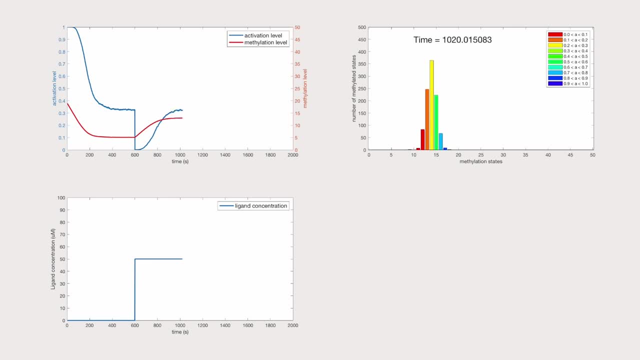 It's shown here in color. It's converging on some universal value. Whenever the level of chemoattractant is being held constant, you get that rainbow color that you see in the graph. Only when the level of chemoattractant jumps do you get a big change in the activation. 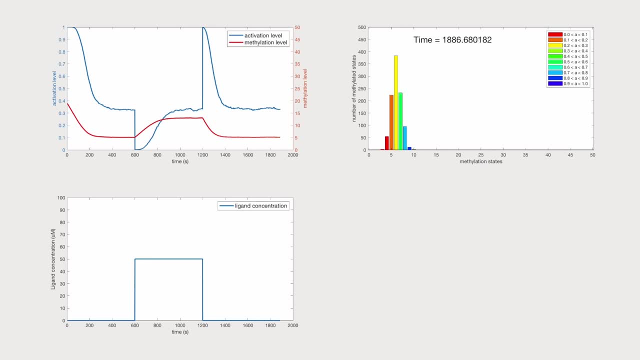 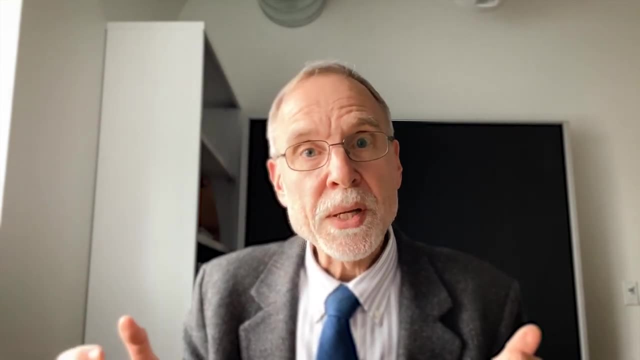 How is that possible? Well, you can also see that in the graph as the bars move back and forth. That's the level of methylation. So by presenting more than one thing at a time in a time series, that enters your brain in a very different way than reading a lot of words on the page, and students find that very powerful. 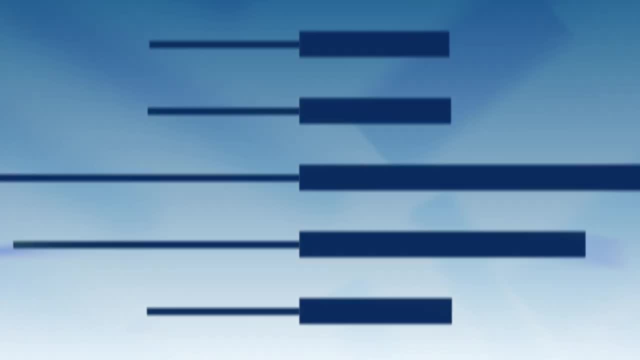 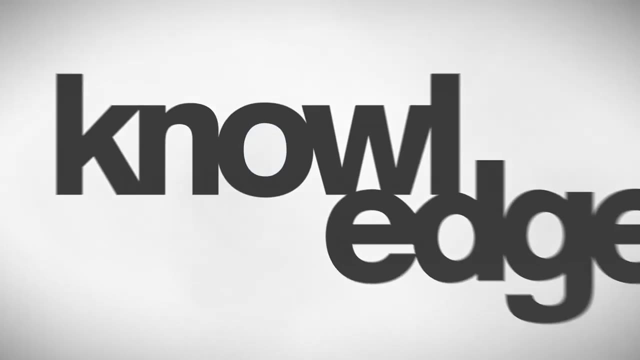 And thank you so much for joining us, Philip Nelson, Thank you.